hello everyone. welcome back to my channel, analytical guy. today, we will discuss about how to analyze sales data using Excel. in my previous video, I discussed on how to create dashboards, so I can show you the dashboard which we created in the last video. if you want to refer to this video, you can click on the 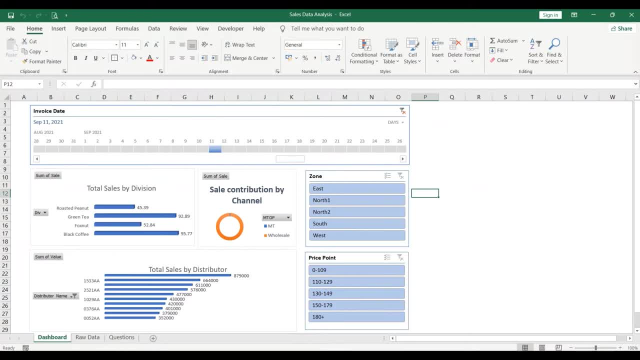 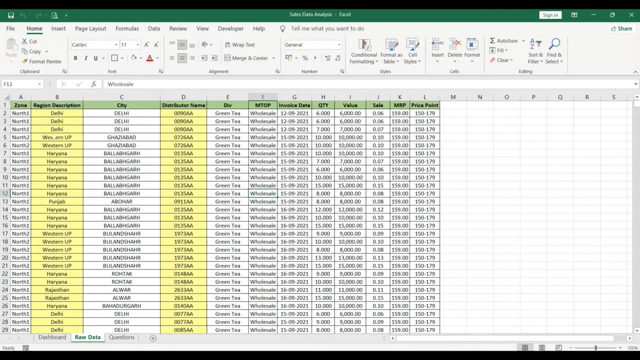 top right screen and you will be redirected to that video. so coming back to our video, so in this video I'll just show you the dummy data. so in this data you can see there is zone. so if, if I filter this, there is north one, north to. 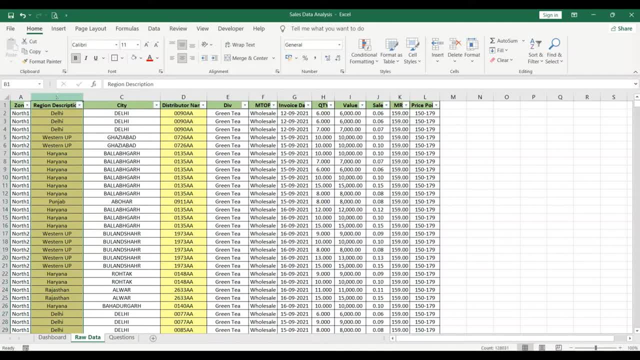 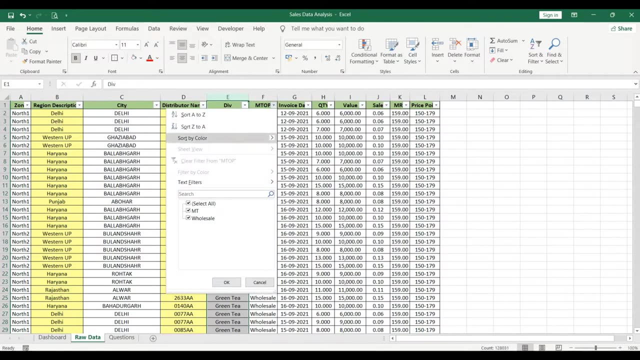 east, south west. then in second column it is region description. you can see the state wise, then city, then distributor name, then there is division. in fifth column there are four divisions in short. then there is a channel in my data. there is modern trade and wholesale, then invoice date- this data is for September 2021- then the number of 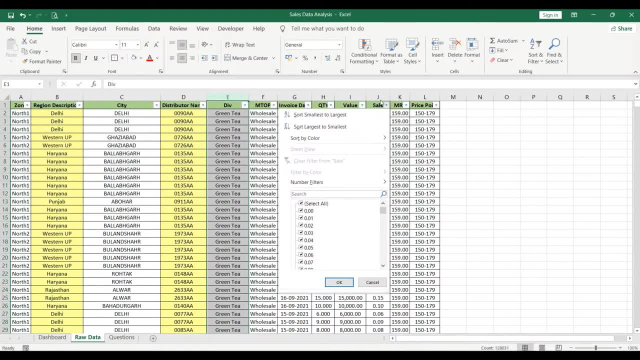 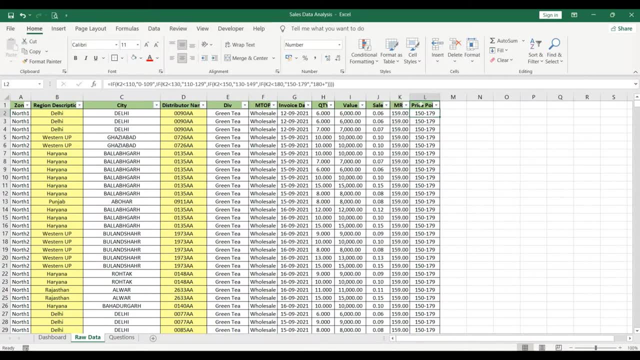 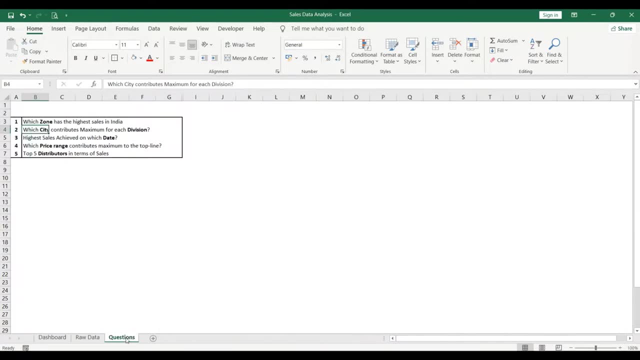 quantity is sold. what is the value? and this sales column is the value in lakhs. then what was the MRP of that quantity? and this is the price point, the range in which the MRP is situated. all right, so our agenda of this video is to answer. 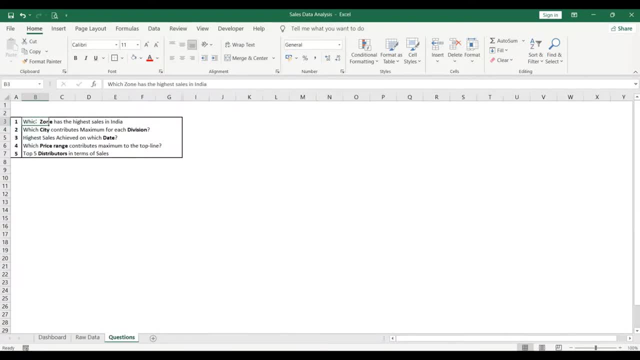 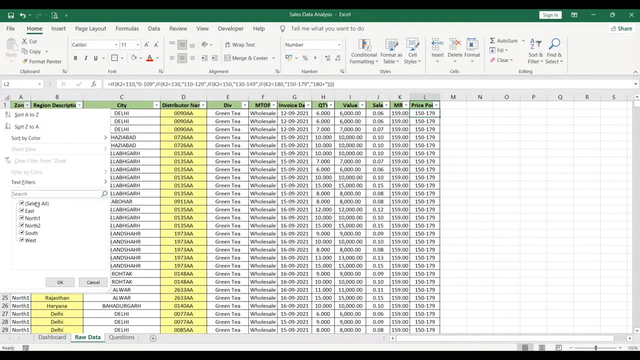 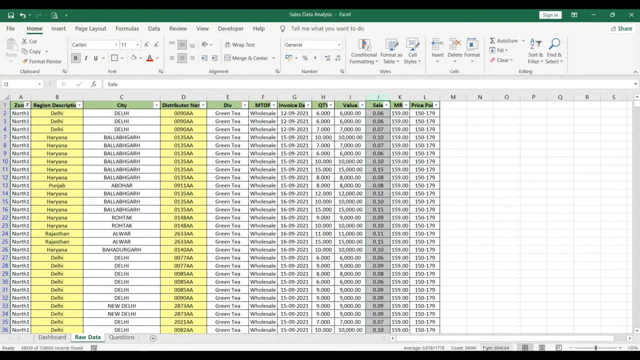 these questions and apart from these questions we'll analyze a bit further. so first question is: which zone has the highest sales in India? so if we have to understand, if you have to get the highest sales, so first you have to filter out. so maybe, for example, in Lehman, you will just say: if I filter north one and just see the sales column, the value. 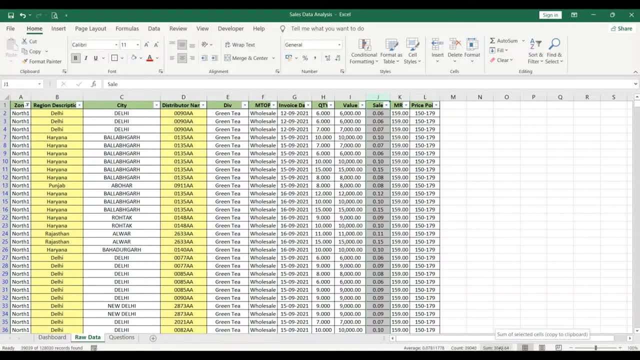 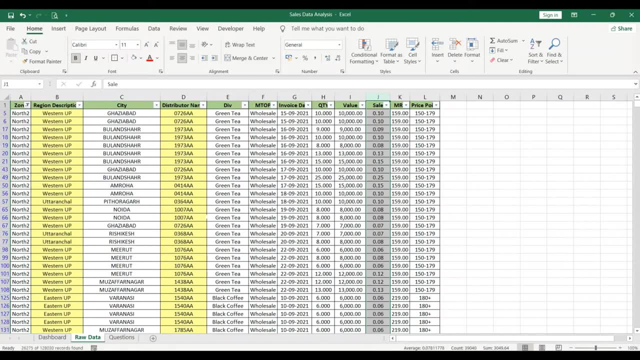 which is coming out to be is 3049, right? so this is north one. so again, I'll go to any other zone, maybe compare and whichever is the highest you will say that's the highest. but this is not at all the right approach, right? so for that, what we'll do is we'll just go to the pivot table first you go to 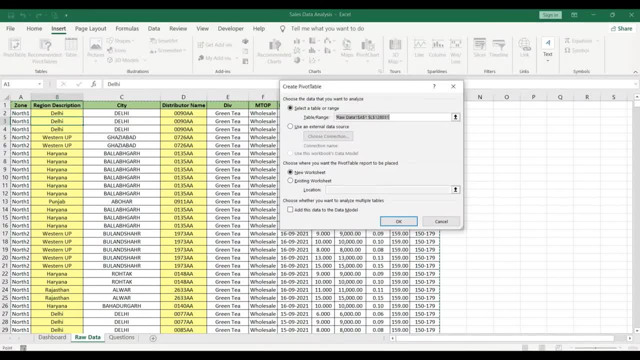 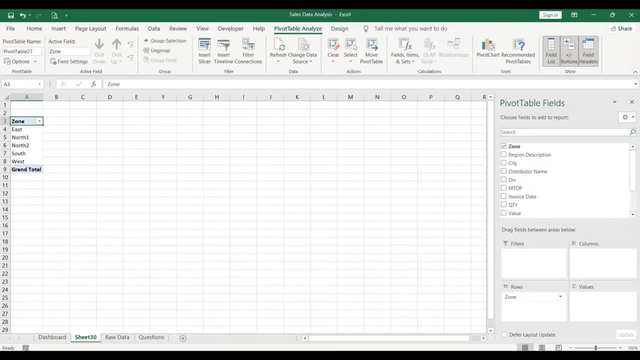 insert, then select pivot table. then there is a dialog box and you'll say, okay, now in this pivot table you will just select the zone and you'll just drag the sales sales. in the value column you can see zone wise sales. so in East the sales was 32,599. similarly, in all these things, if I 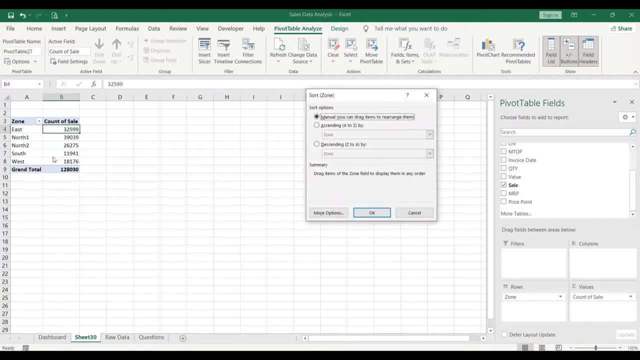 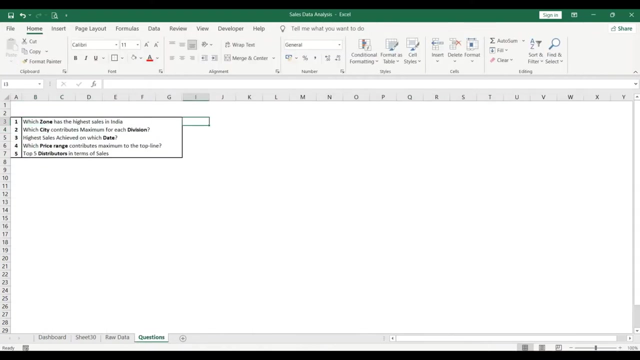 have to fill, sort it out, so I'll just go to more sort options. I'll just do descending z2a from count of sales. okay, so now you can see the highest sales was in north one, correct, which is thirty nine thousand thirty nine. so answer for this question is third north one, north one. all right, so you have answered one question. 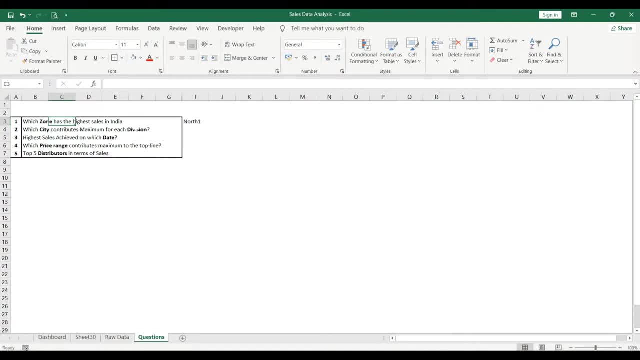 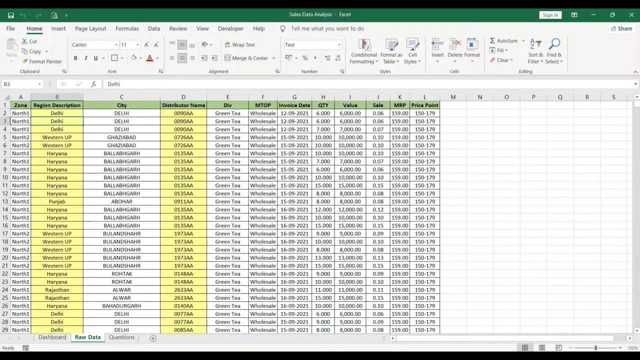 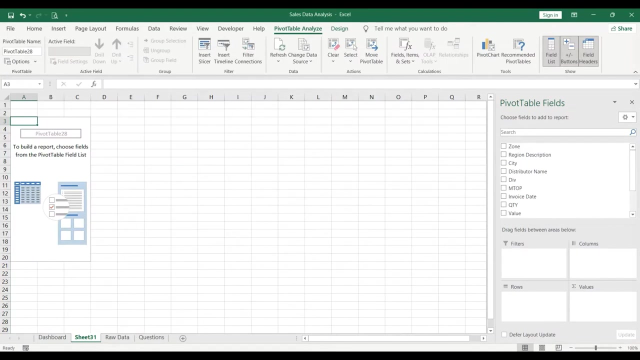 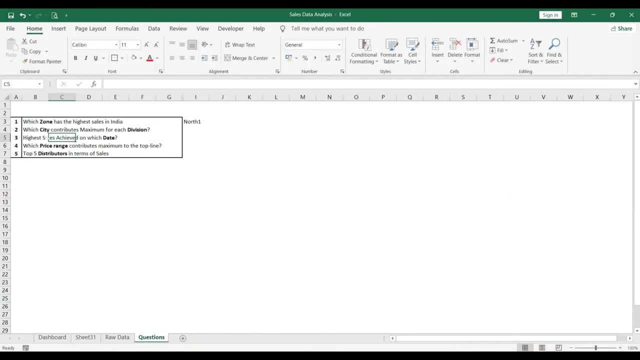 second is: which city contributes maximum for each division? all right, so each division with city contributes maximum, all right, all right, so to answer this question will again go to pivot insert. then we were table select- okay, all right. so now here we have to select all the cities that can go into the row, so you have to see which city contributes maximum for. 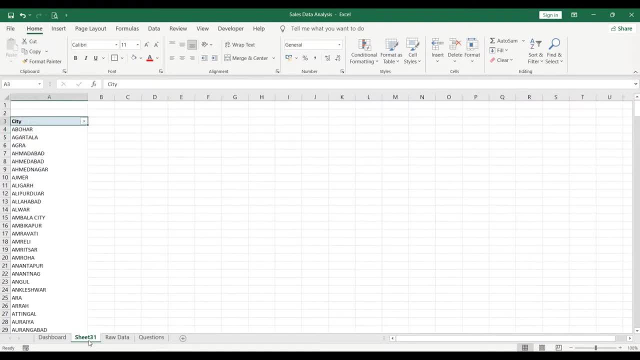 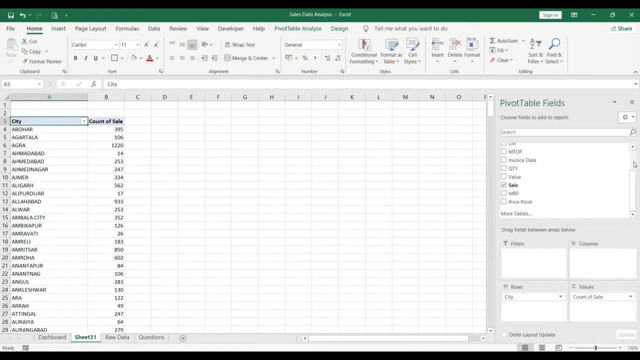 each division, right, so now you have selected city. now you have to select the sales as well. so sales you can drag to the, the, the, the and you have to do this filtering through division. right, so you can add, add a slicer of division. so you right click to the division and add a slicer, all right. so if 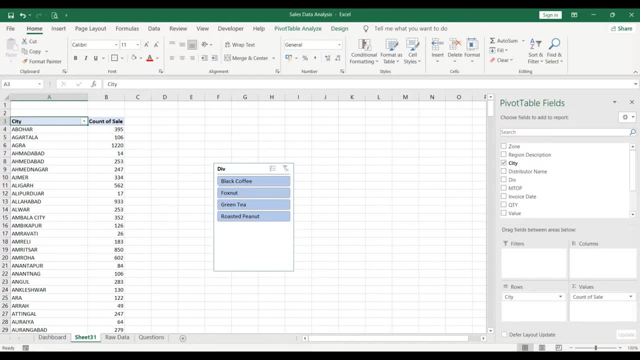 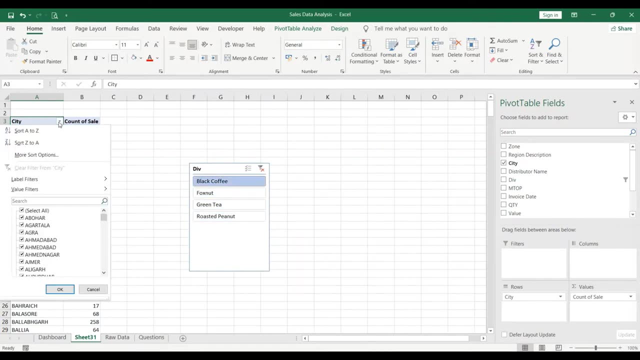 you have to understand which city contributed maximum for, let's say, black coffee. you just select on black coffee and you will see. okay, so i'll just sort it out in descending order to count of sale, right? so if i selected black coffee, you can see delhi is the highest contributor. 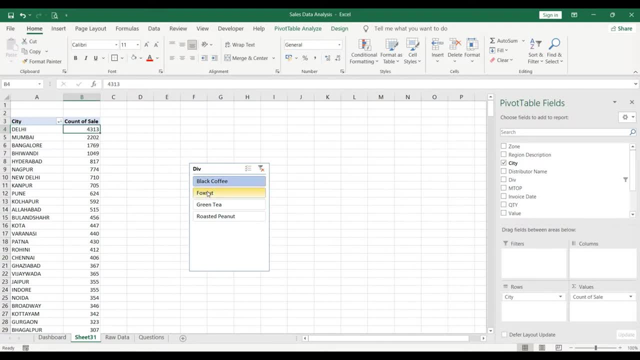 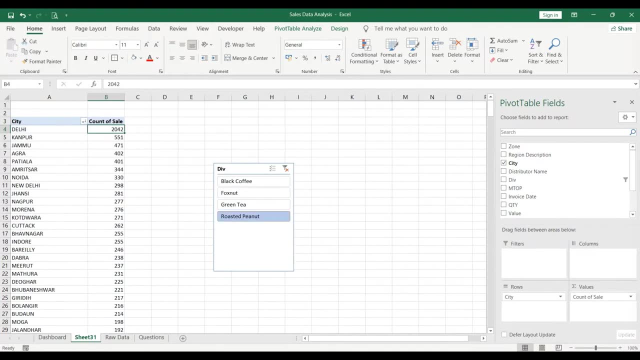 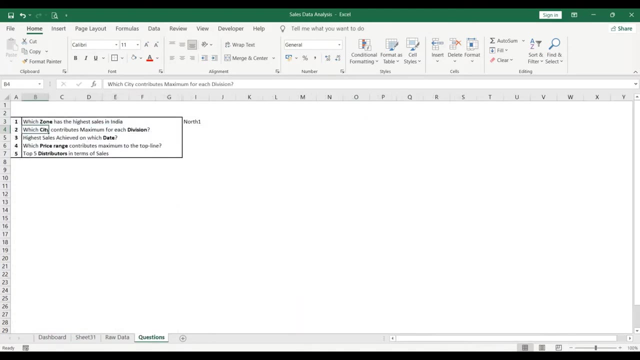 by uh, with four, three, one, three right, if i select. fox nut, again delhi is there. in green tea also, delhi is the highest seller. and roasted peanut, again delhi. so in all four division, delhi is contributing the maximum. so the answer to this question would be delhi. 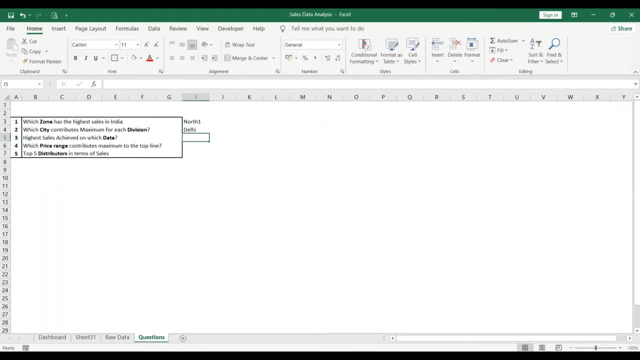 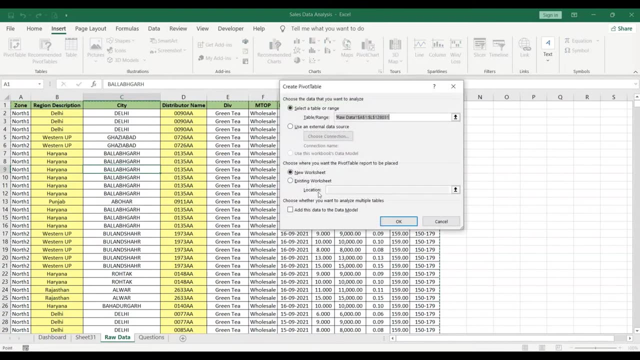 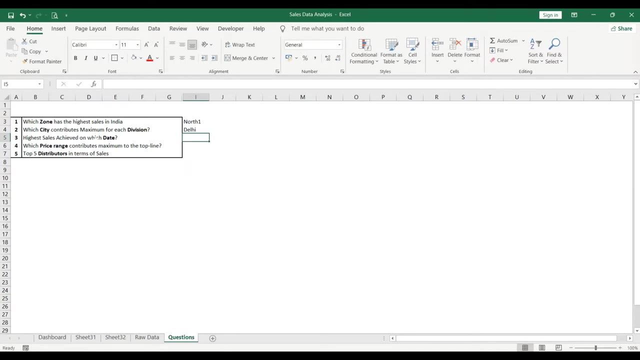 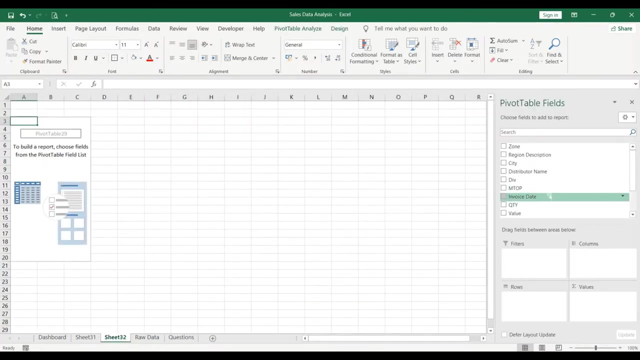 now coming to the third question: highest sales achieved on which date? so again you go to the raw data, insert pivot table and you click ok. now the question read again: highest sales achieved on which date? so you have to add date column and sales. so invoice date can go into the rows right and sales value can go into the values. 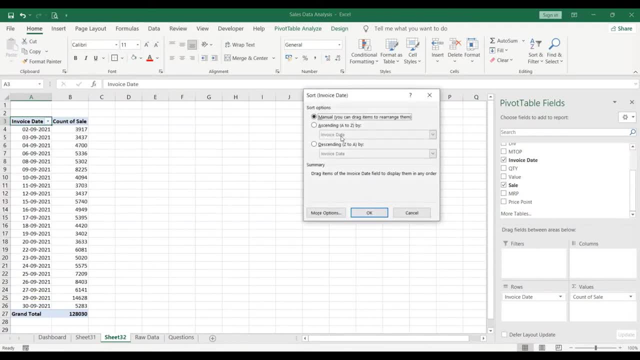 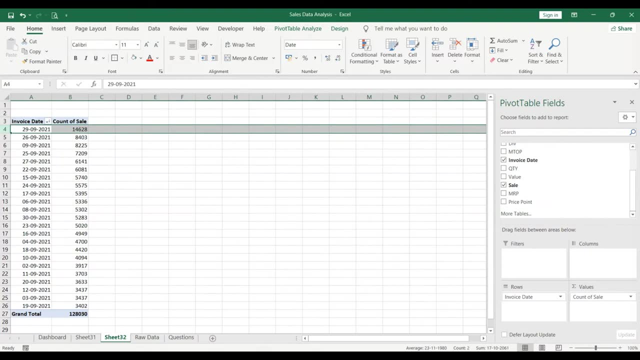 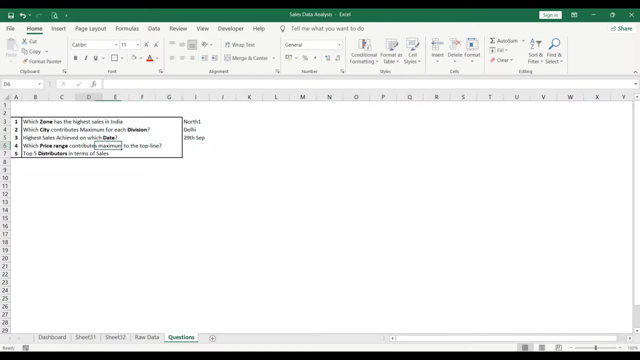 and again, if you sort it out in descending order through count of sales, you will see which date contributed the maximum. so 29th september contributed 14 628 sales, right? so answer would be 29th, 29th september. so fourth question is: which price range contributes maximum to the top line? 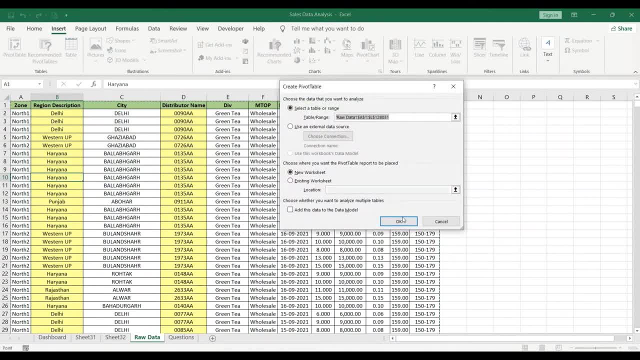 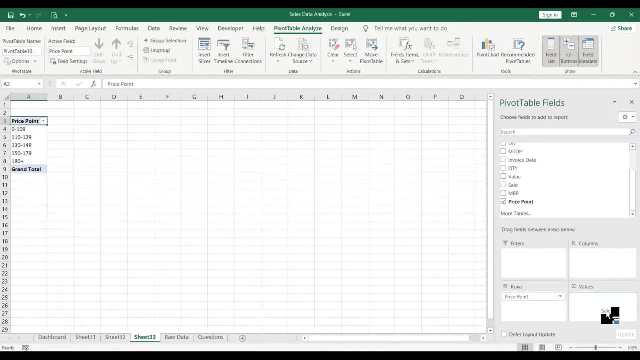 all right. so again, we'll just have another pivot table. all right, so this time i'll just select price point in rows and then sales in value. all right? so see, top line is equivalent to revenue, which is sales. right? so again, i'll just sort it out. 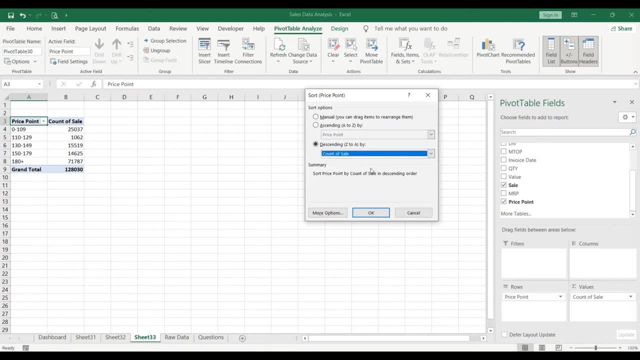 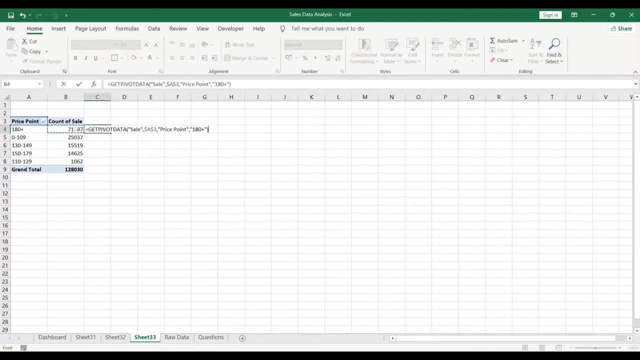 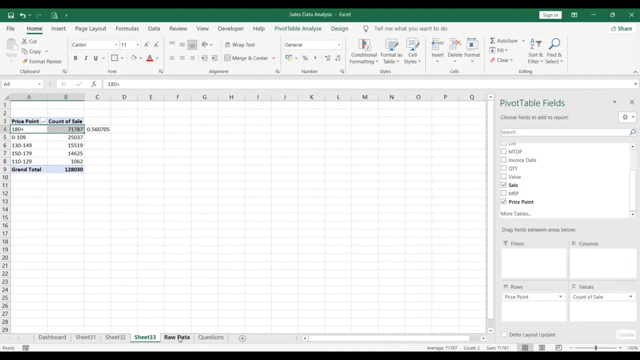 out in descending order of count of sale, right? so in this 180 plus price point is contributing 71787 out of one lakh twenty eight thousand thirty. so this is almost what percent? 56 percent it is contributed, right. so the answer for this question is 180 plus. 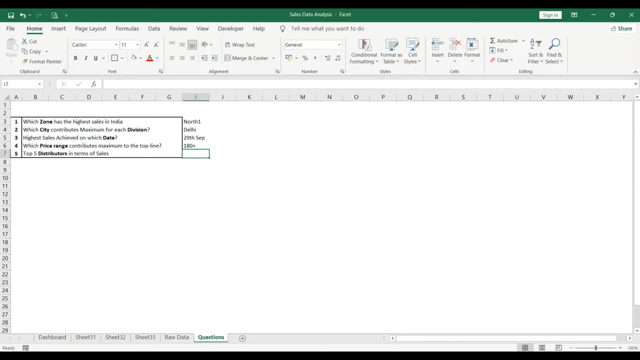 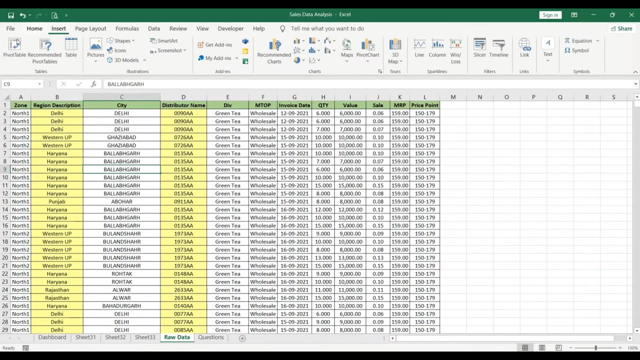 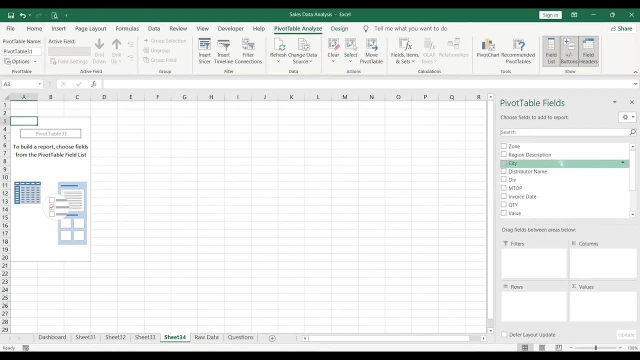 we have answered four questions. our last question is top five distributors in terms of sales, which are my top five distributors. so for that again i'll just insert pivot table so you can understand the importance of pivot to analyze the data right. so here i'll just get the distributor. 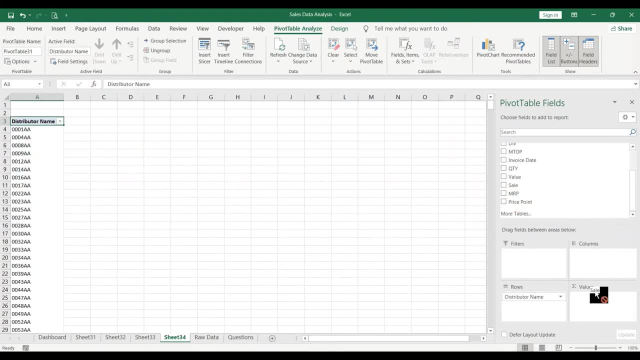 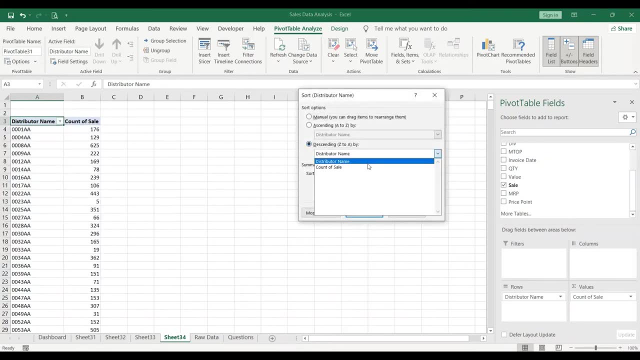 names and select sales into the value column and again i'll sort in descending order of count of sales, right, and from here i'll just do value filters. in top 10 i'll select 5 right, and then okay. so you can see these are my top five distributors. 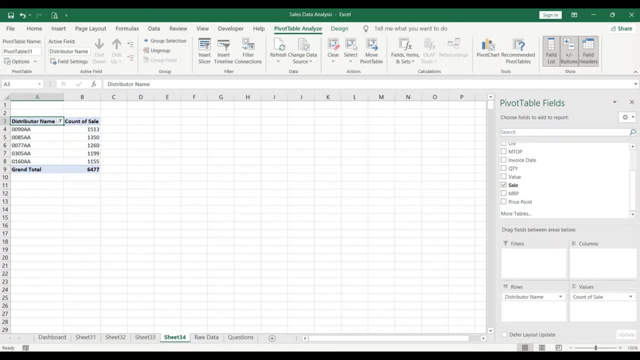 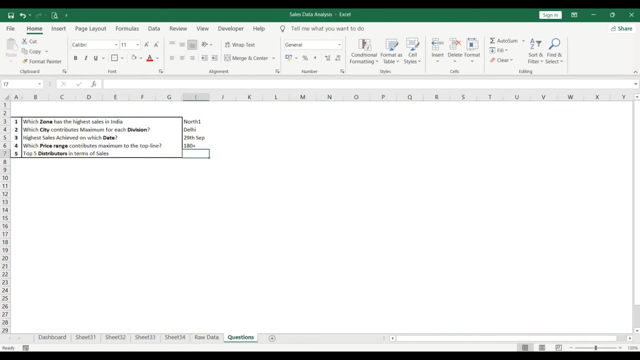 uh, who are contributing to my top line. so this is zero, zero, nine, zero aaa. and then, like, these are five distributors, right, so these are our top, these are my top five distributors, all right, so now we have answered all these five questions. so, uh, there's one more thing which i want to mention in uh pivoting. so, for example, if you 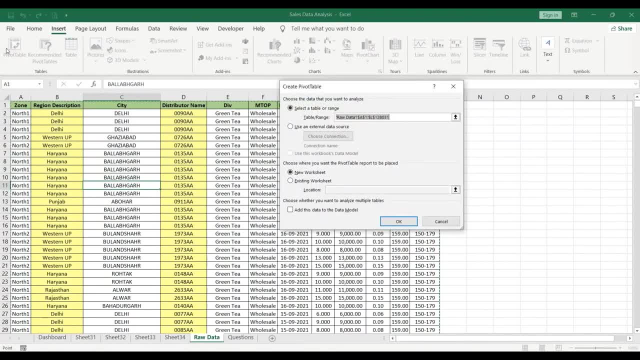 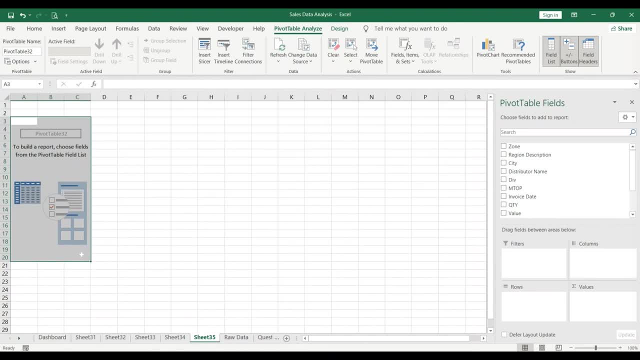 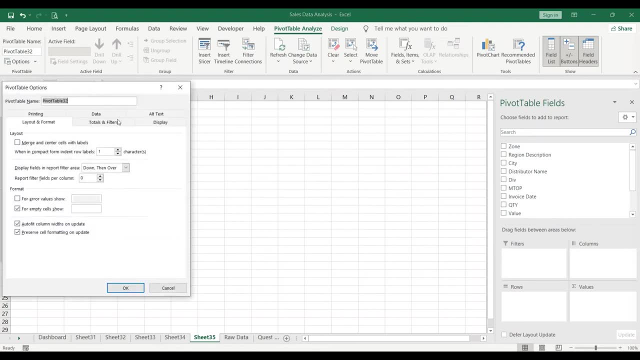 go to this table, you insert pivot table and you click okay, so you get this kind of grid right. so this grid is usually not recommended, so you want to have another grid. so, uh, where you do right click, you go to pivot table options, then you do display and then you take classic pivot. 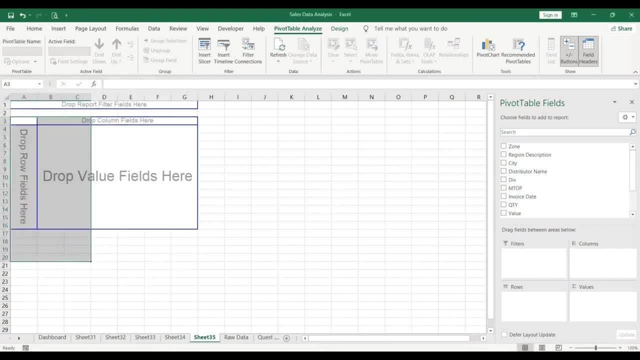 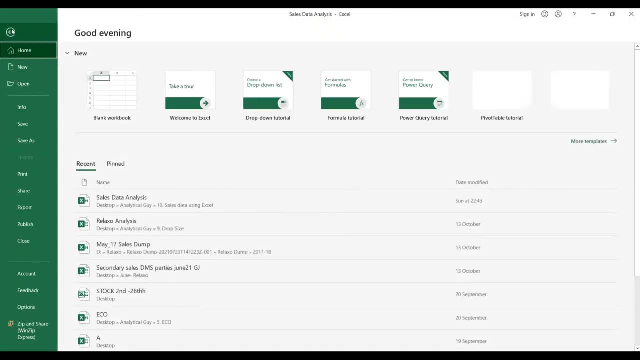 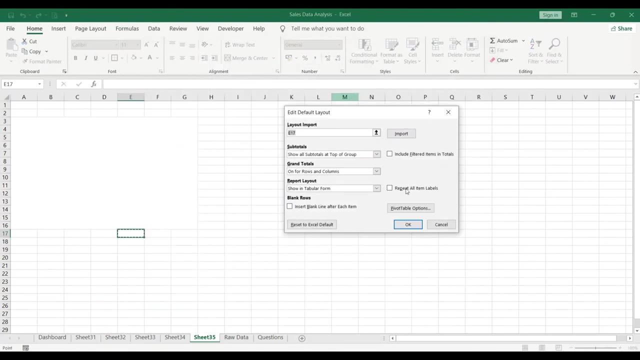 table layout. so you want classic pivot table layout in general, right, this kind of layout. so how can you make it as general, right? so if you go to the file, go to options, uh, you select data and edit default layout. and if you go to the pivot table options, 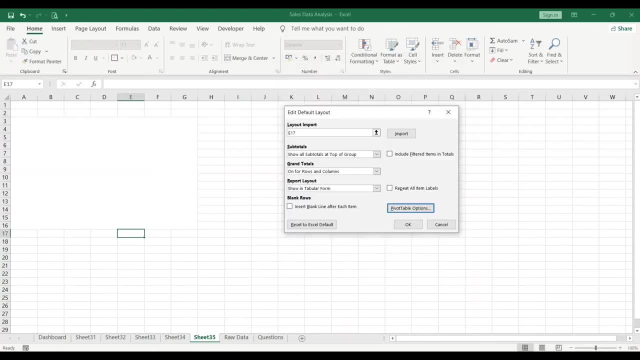 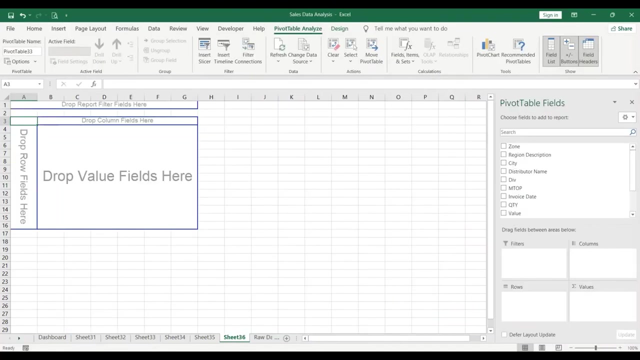 you click classic pivot table layout, okay, and then you again click ok, so this is now a default feature now. so again, if i go to a raw data, insert pivot table now you can see the difference right. so this is one of the hacks which you can easily use, for example now, if you. 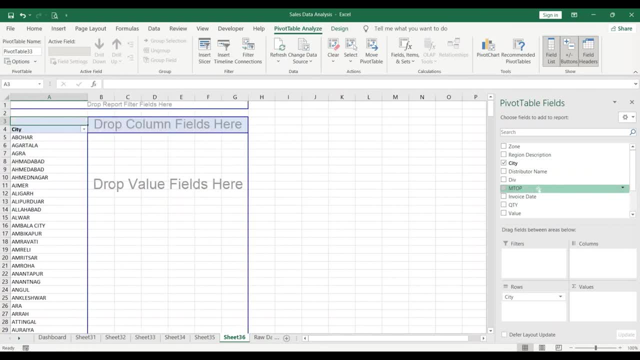 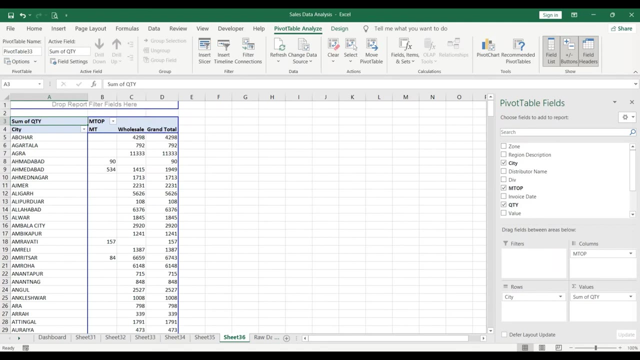 have to drag city in rows, you can directly do that. then if you have to insert the channels in rows, you can do that. then if you want to add input quantities in drop value fields, you can do that. so it is quite easy to play with the data in this regard. right, all right. so this is it in this video. 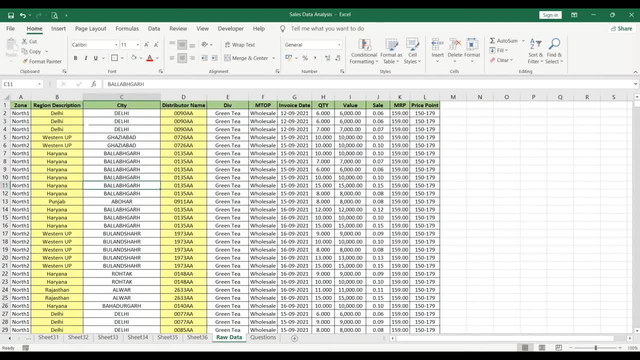 so if i go back to my raw data, you can see you can analyze geographically, you can analyze division wise, you can analyze channel wise, then you can analyze quantity wise and sales wise as well. so if, given the data, you can analyze any kind of analysis, all right. so you have answered all these.